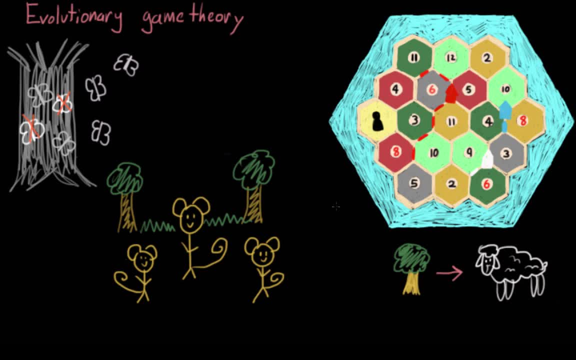 So let's think about this in terms of game theory, where life is the game. What strategies would you expect to see from the players? Well, like in Settlers of Catan, you would expect them to be concerned with the availability of their own resources. 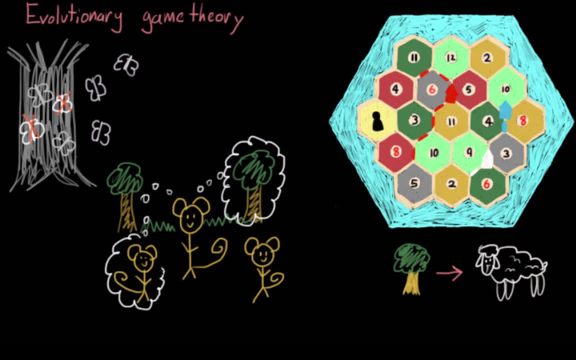 But you would also expect them to be concerned about their social behavior, since so much of their well-being and chances of mating rely on their interactions with others. And this is exactly how evolutionary game theory fits in with general game theory, Because the strategy of each individual will depend, at least in part, on the strategies exhibited by the other players. 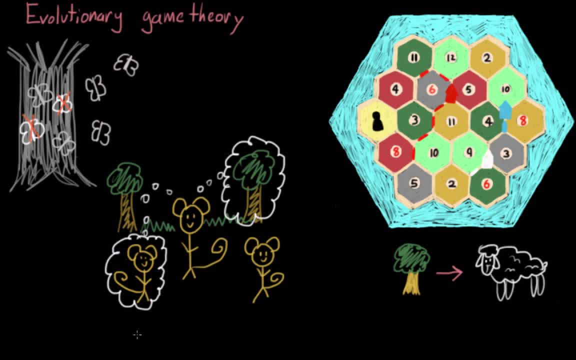 I do, however, want to point out a big difference between evolutionary game theory and general game theory, Because game theory generally involves intention or cases where individuals are actively reasoning about the strategies or the behaviors of other individuals. Evolutionary game theory is different because it is applying this theory to situations where there might not be any overall conscious intention on the parts of the players. 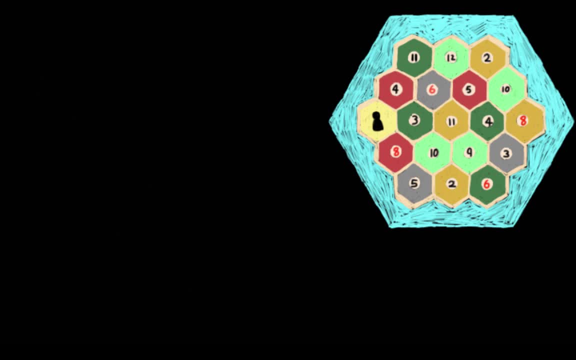 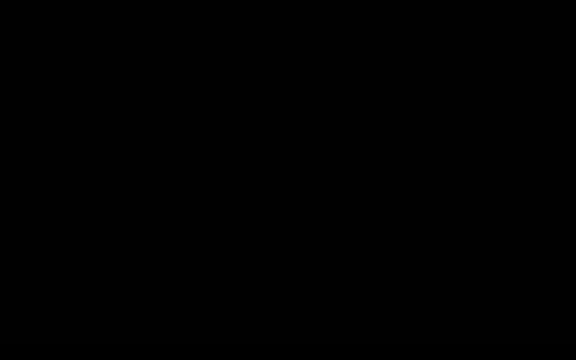 Another thing that I want to point out about evolutionary game theory is that it can actually help us predict the traits we would expect from other players. Evolutionary game theory predicts the appearance of evolutionary stable strategies or behaviors that tend to persist within a population once they are prevalent. 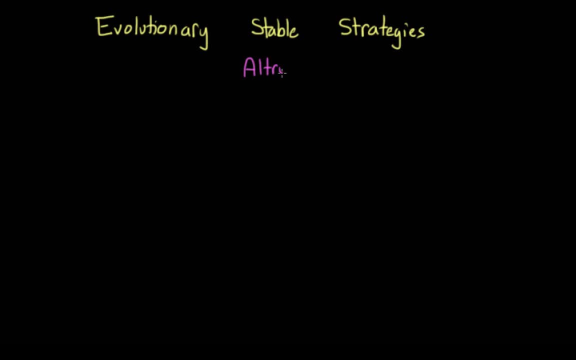 So let's think about this in terms of a complex behavior like altruism. So imagine that we have two groups of monkeys. In one group, the monkeys act selfishly When one sees a predator approaching, he takes the time to hide and does not warn the others. 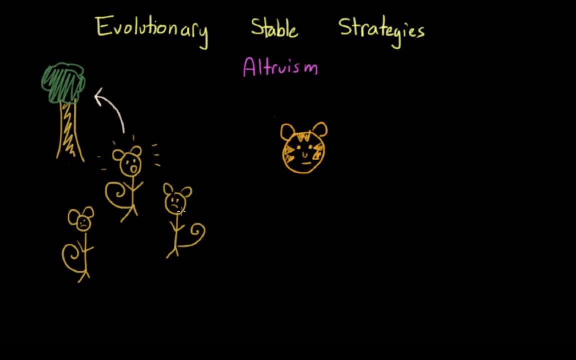 Which makes it more likely that he'll escape and that the predator will eat one of the other monkeys instead. And now, on the surface, it seems that this is a pretty good strategy to ensure survival. After all, you get out of it alive. 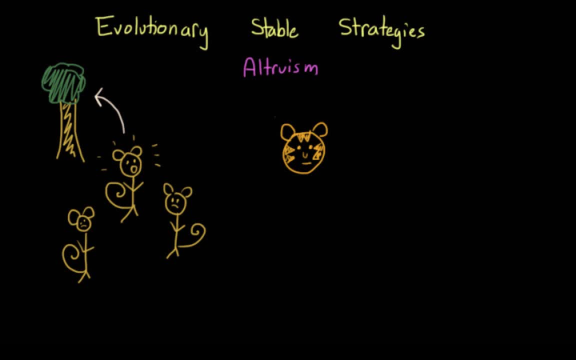 However, imagine what would happen if the entire group behaved this way. It would mean that our monkey would be more likely to die if another monkey also didn't sound the alarm, And over time this could decimate that monkey population and reduce the fitness of the overall group. 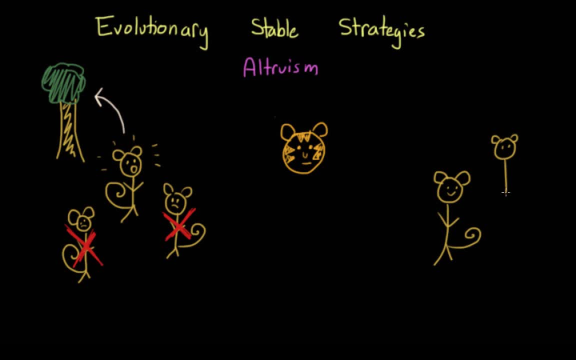 But what if they adopted another strategy, one that involves giving an alarm call whenever a predator was spotted? The monkey that would make this call is doing this at any time, At his or her own expense, because it could draw the predator to them. So initially you might think that this strategy would fail.